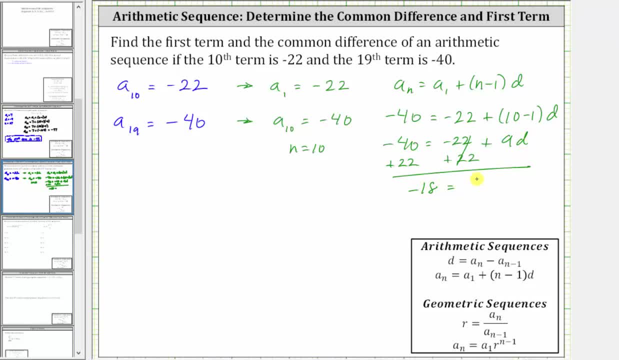 Simplifying, we have negative 40 plus 22,, which is negative 18, equals nine. d Solve for d. we divide both sides by nine And simplifying, we have d is equal to negative two. So now we know the common difference d. 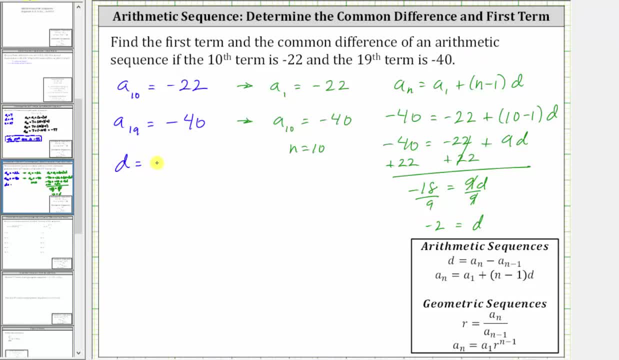 for the arithmetic sequence is negative two. So now we can stop pretending and go back to the original sequence and determine the first term. So again, our goal here is to find a sub one with this given information. So again, using the formula a sub one. 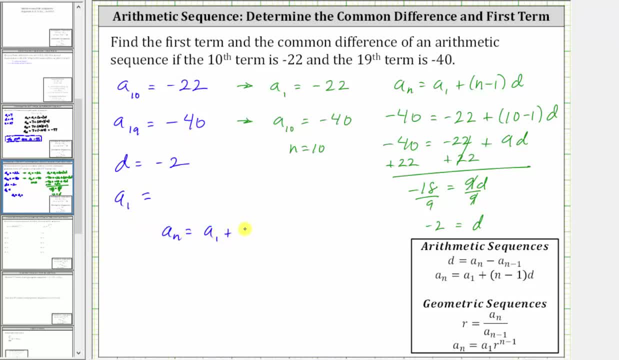 and using the formula, a sub n equals a sub one plus the quantity n minus one times d. we need to decide whether we want to use a sub 10 or a sub 19 for a sub n. Let's go ahead and use a sub 10.. 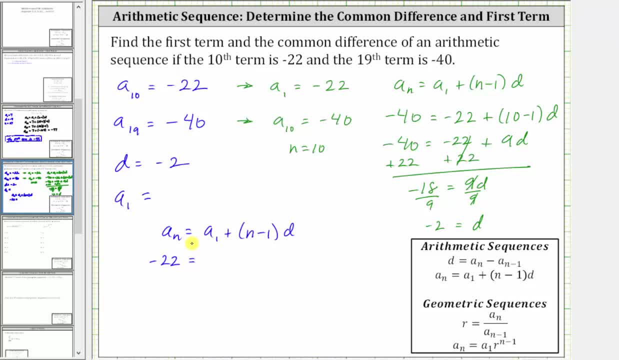 So if we substitute negative 22 for a sub n, we now know that n is 10.. So we know negative 22 must equal a sub one plus the quantity 10 minus one times the common difference d which we now know is negative two.